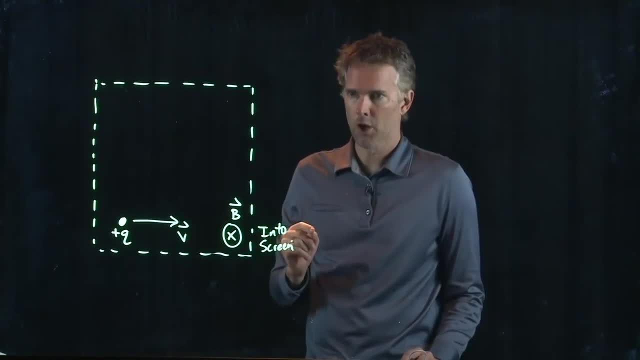 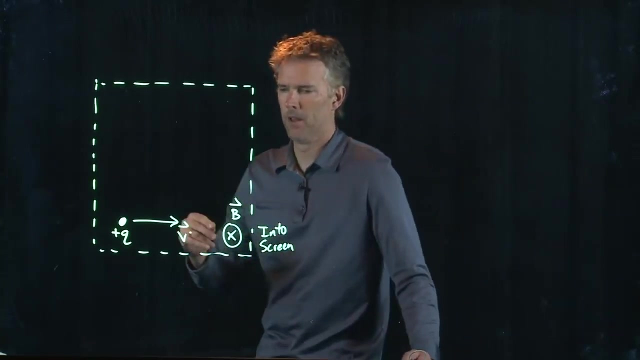 fingers straight in the direction of V, curl them into the screen for the direction of B. Which way is the force? It's got to be up or down. What do you guys think Anybody get an answer on that one. Let's try it. V is going to the right, B is into the screen. 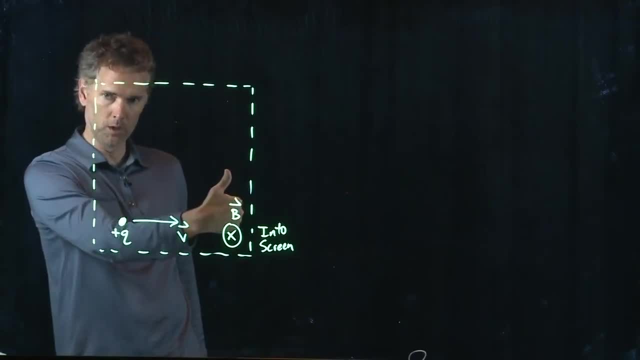 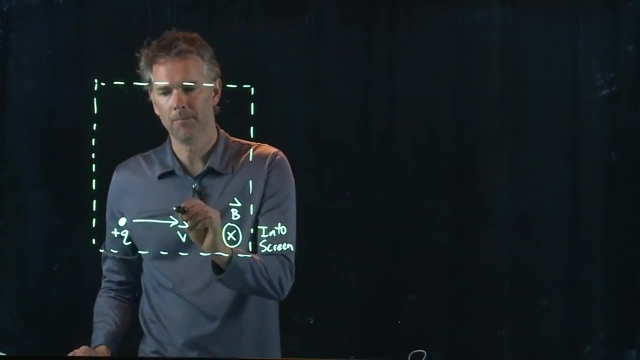 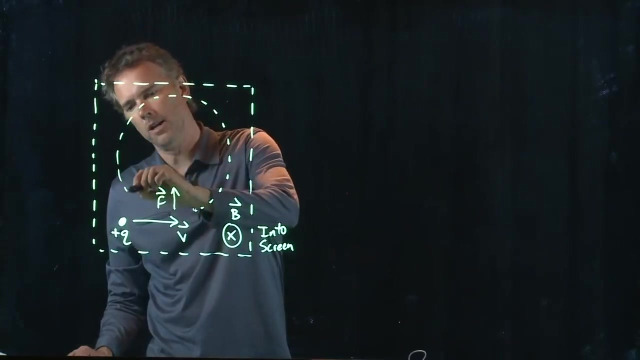 So I'm going to curl my fingers into the screen, right? That's to you what looks like into the screen, okay, And so I'm going to end up with a force that is up and that means that this thing is going to move in a circle. 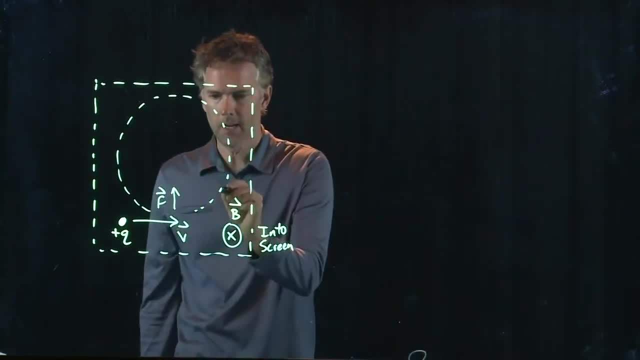 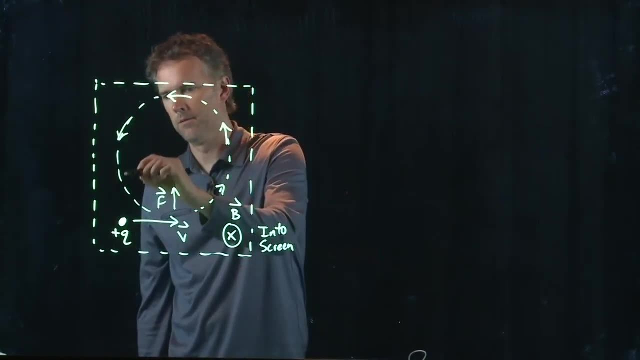 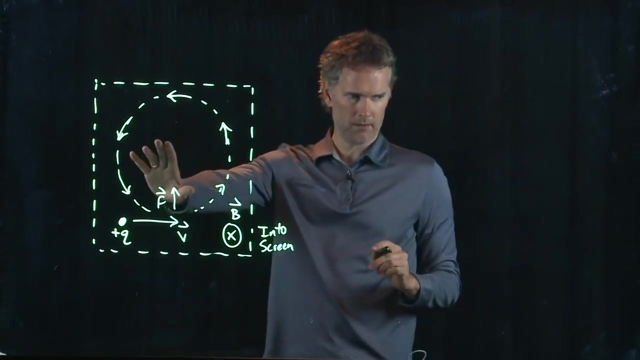 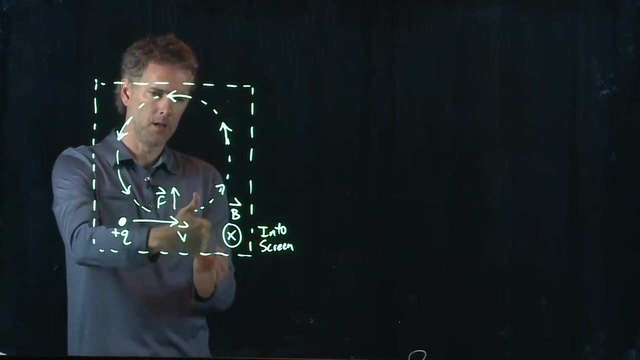 Okay, and that particle that came flying in is in fact going to move around in a circle. Okay, is that right? Did everybody see that? Okay, V is to the right, B is into the screen, Thumb is the direction of force, So it's towards the center of the circle at this point. Well, 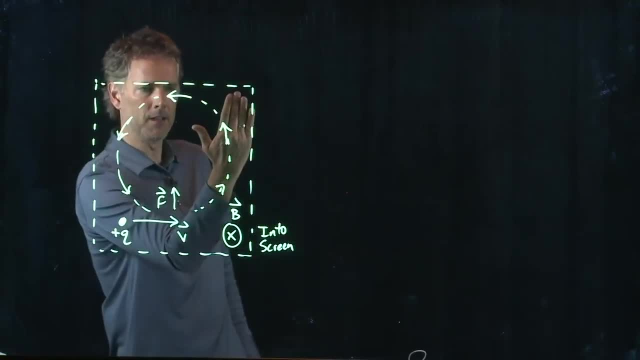 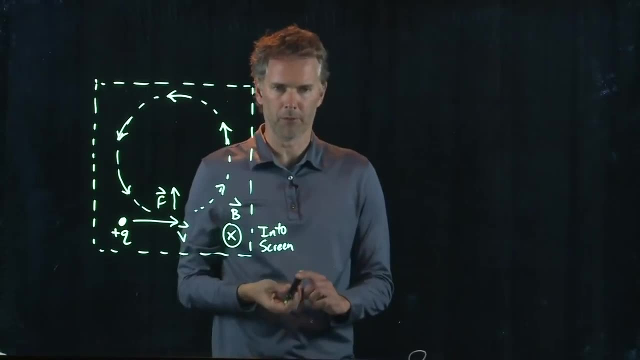 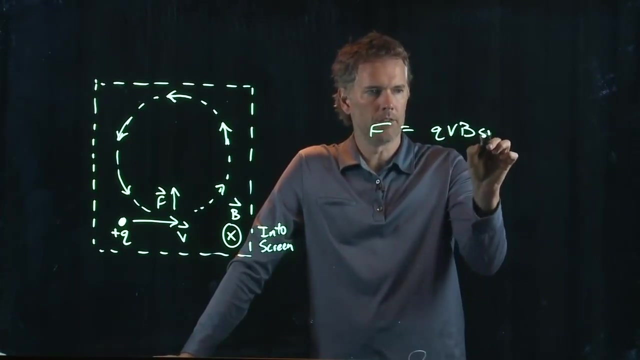 later on, V is going up, B is into the screen, And so I again get a force towards the center of the circle, And everywhere around it's always a force towards the center of the circle. Okay, but we know what that force is: It's qVb, sine of theta. Let's just worry about. 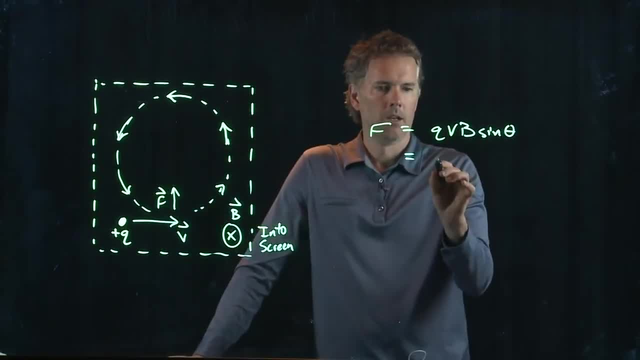 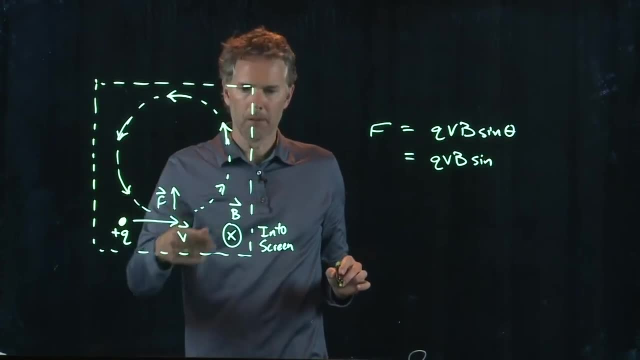 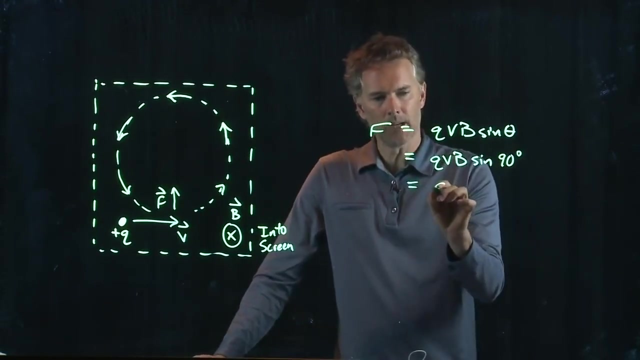 the magnitude of it. We've already figured out the direction qVb. What's the angle between those two? QVb was to the right, B was into the screen, and so we get 90 degrees. but 90 degrees is just one. 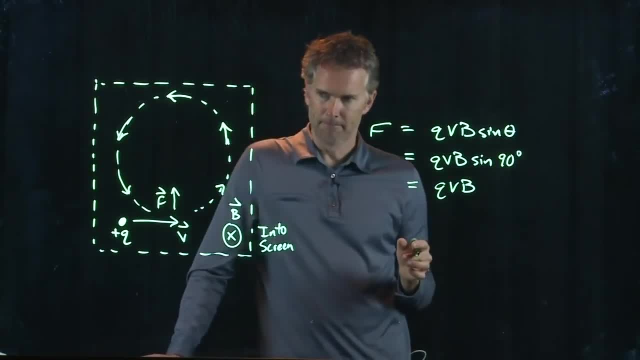 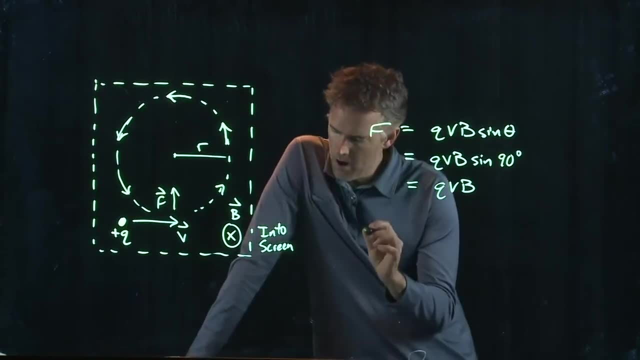 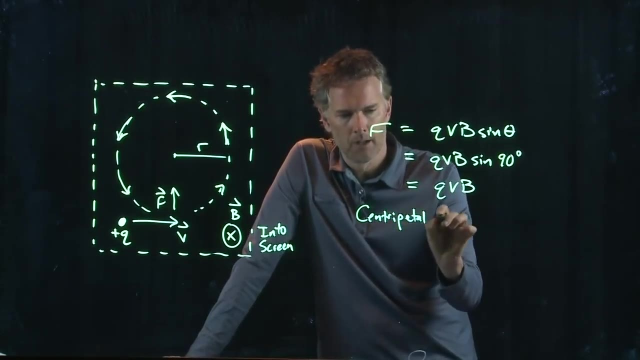 So what's the force? QVB, All right, but this thing is moving in a circle now of radius R, and what we know from last semester is: if things are moving in a circle, we can consider the forces adding up to something very specific. 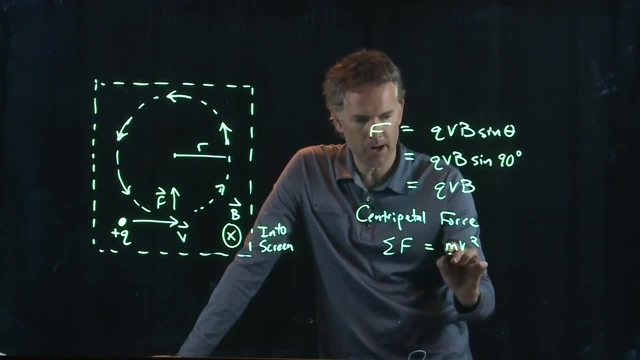 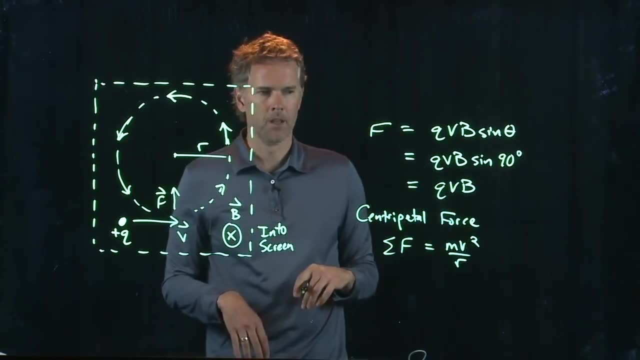 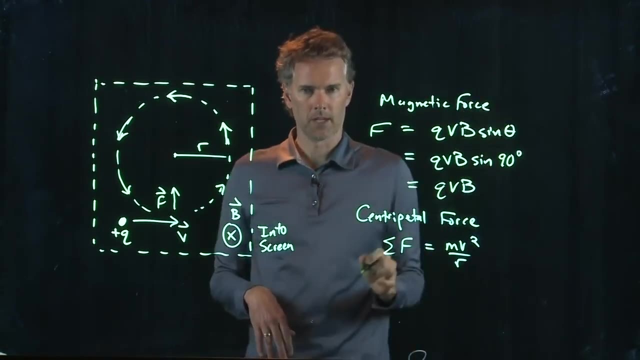 namely mv squared over R. right, This is uniform circular motion. The centripetal force is mv squared over R, but the only force is this magnetic force. okay, And so that becomes the left side of this equation. So we get QVB. 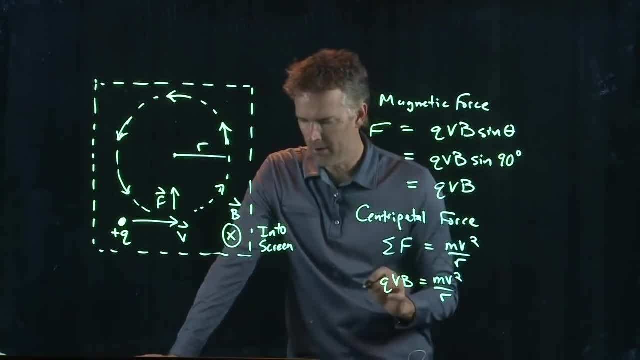 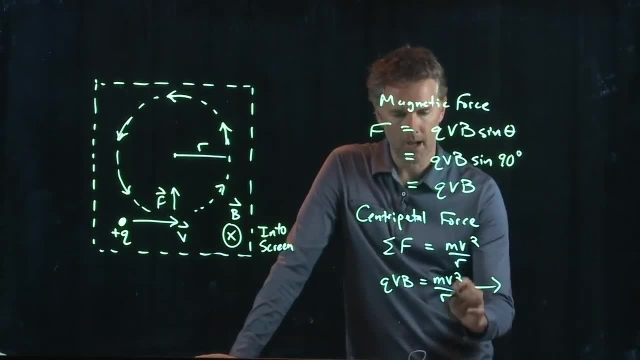 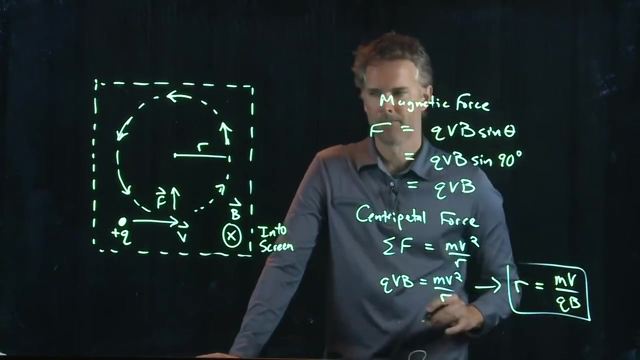 equals mv squared over R. And now we can quickly solve this thing. for the radius right, I multiply by R, I'm going to divide by QVB, One of the v's is going to cancel out and I get mv over QB. okay, What's the radius of that circle? It's that. 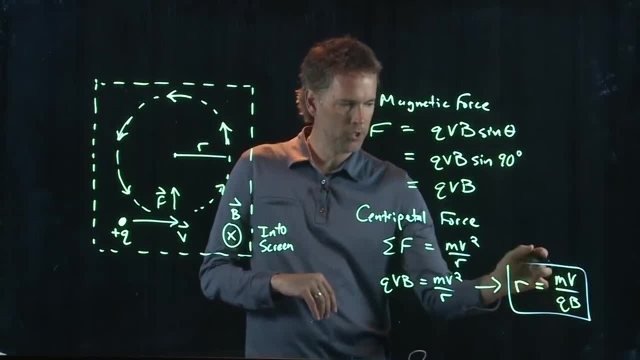 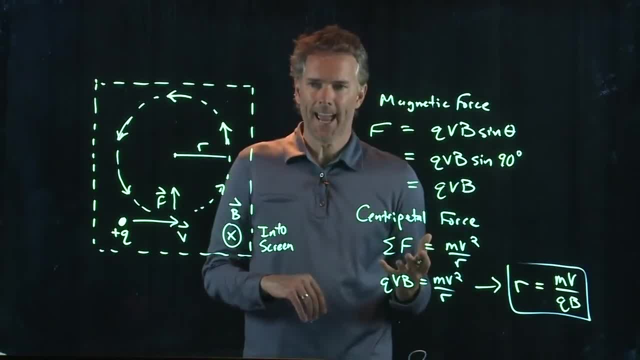 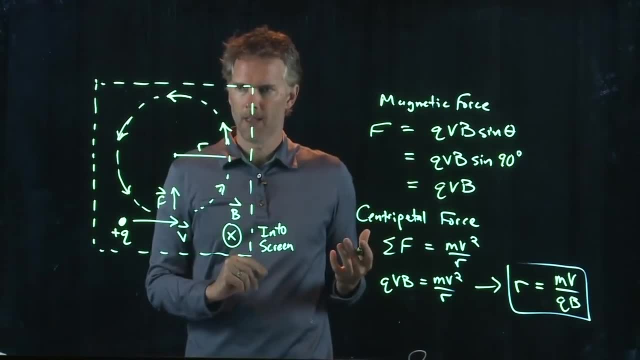 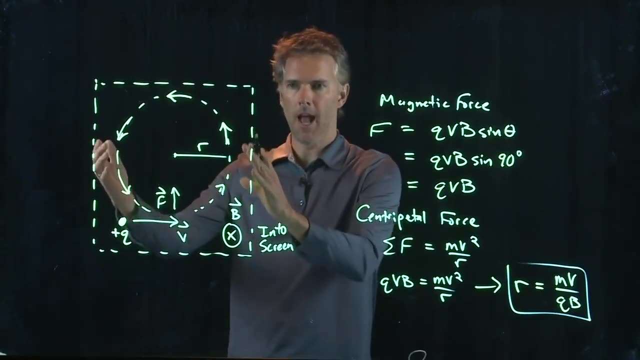 So when you are doing a high-energy physics experiment and you create all these charged particles that are moving very quickly, how can you determine something about them? Well, you put them in a big magnetic field and you watch them spin around in a circle, and when you do that, you can determine this quantity right here. 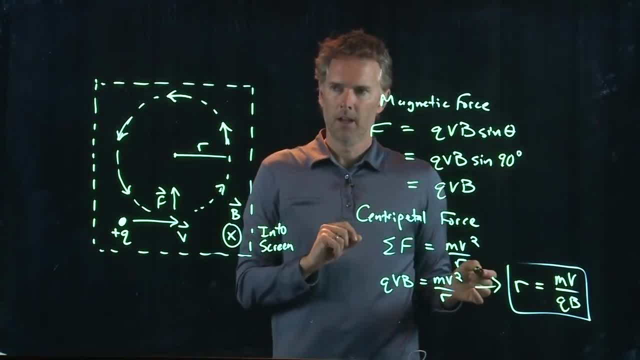 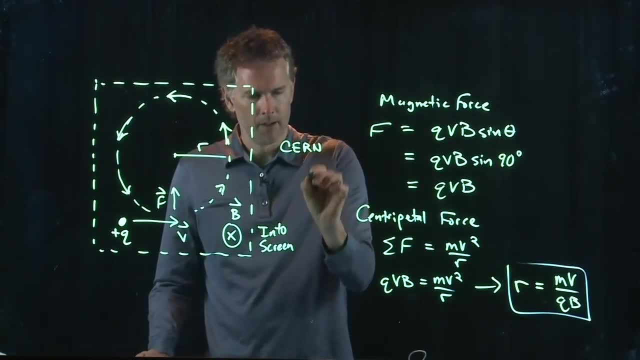 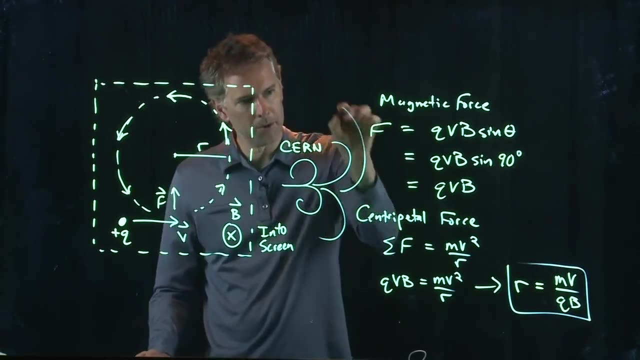 you have to do is determine the radius of the circle. And so when you see those pictures from CERN and places like that where they have particles coming in and then doing this sort of stuff and this sort of stuff and all these circles and beautiful pictures like that, what those are are charged particles moving through. 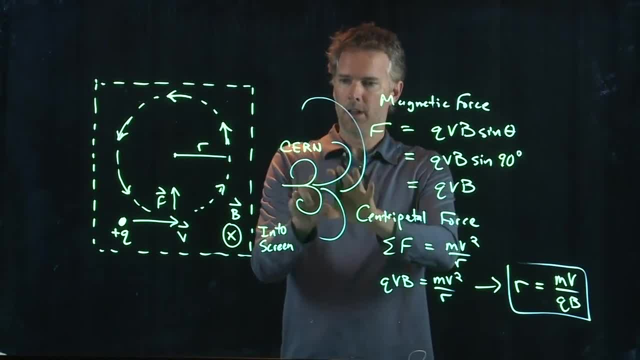 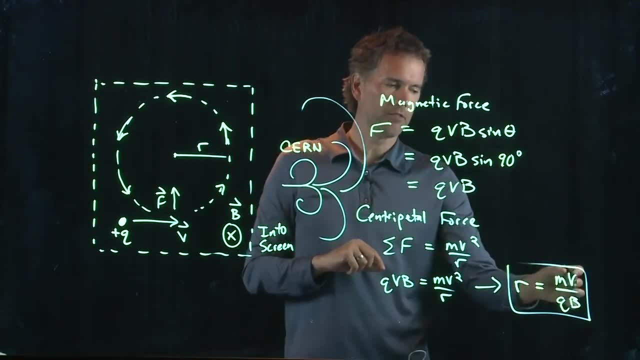 magnetic fields And from those pictures all they have to do is measure the radius and if they know the magnetic field that was in there, they can figure out something about how fast it's moving. What's the mass, What's the charge on it? 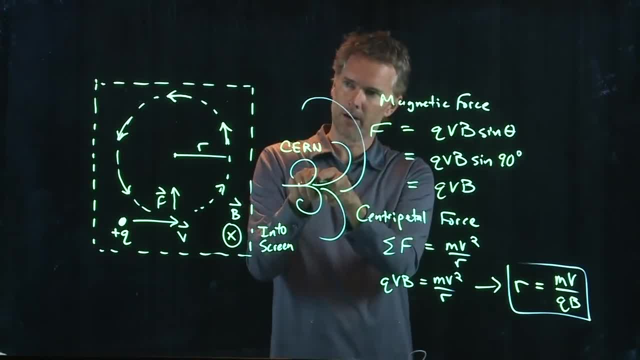 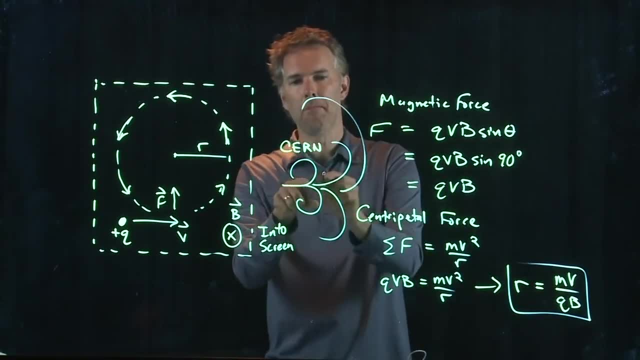 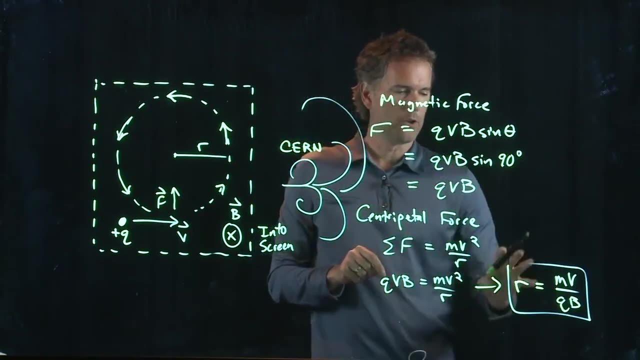 Positives are going to go this way, Negatives are going to go the other way. Okay, Ones that are very lightly charged have a small cube, have a bigger radius. If they have a bigger mass, they have a bigger radius. Okay, And so you can.